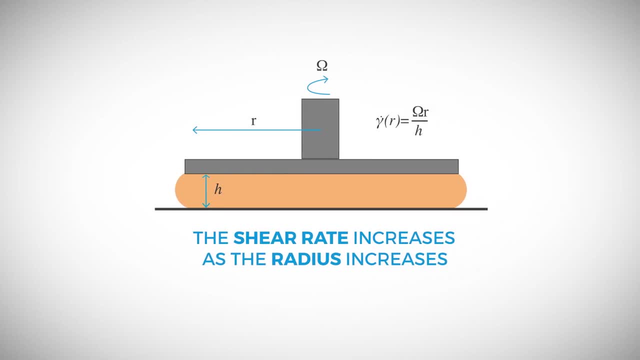 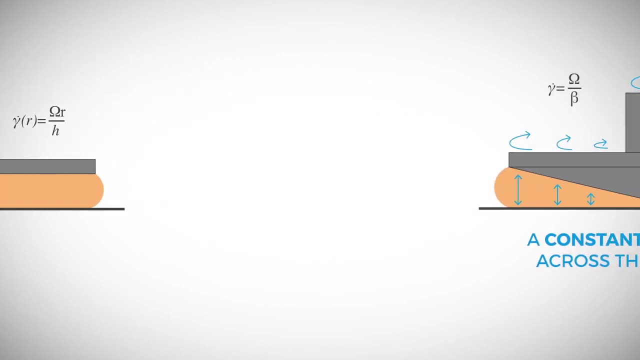 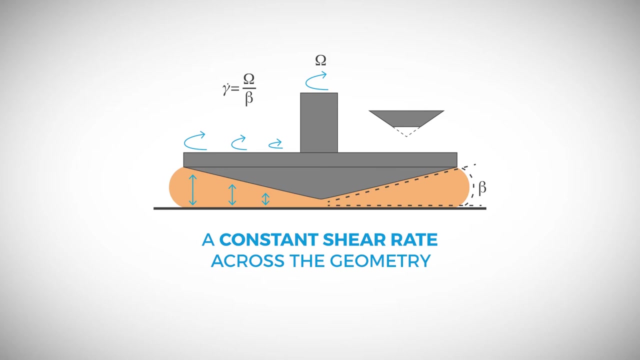 differences to consider. One difference is the shear rate in the radial direction. For parallel plates, the shear rate increases as the radius increases. For cones, the chain in slope results in a constant shear rate across the geometry. The constant shear rate makes the cone and plate useful for measuring normal stresses. 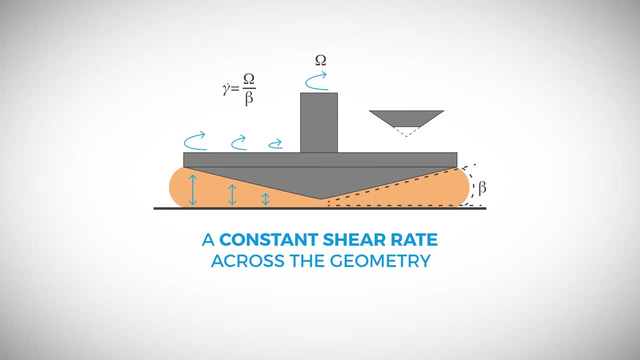 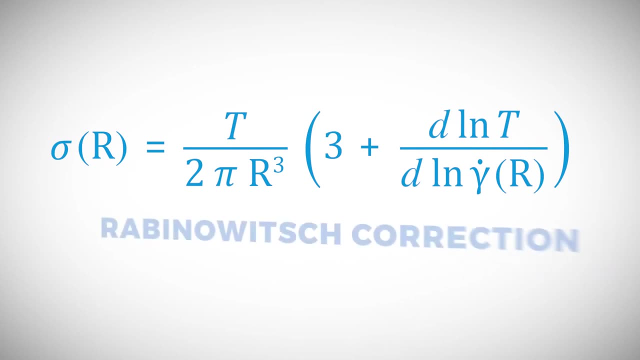 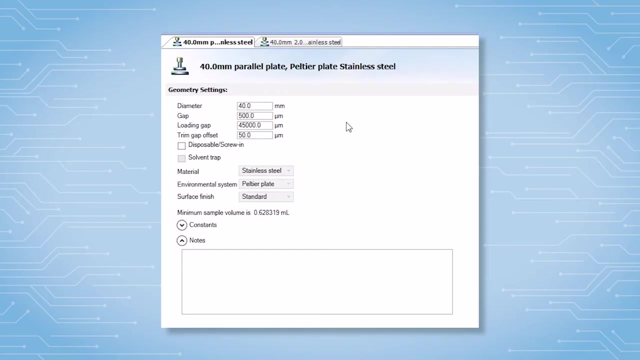 Additionally, cones accurately measure the shear viscosity as a function of shear rate, Due to the change in the shear rate in the radial direction. for parallel plates, the viscosity of non-Newtonian fluids may be corrected using the Rabinowitz correction. During temperature ramps, the geometries expand. 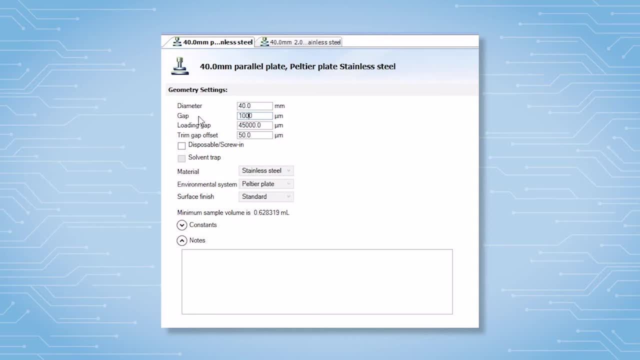 as the temperature increases, based on the coefficient of thermal expansion. Parallel plates are preferred in this case because they can be operated at a variety of gaps. The operating gap for cones is the specified truncation gap. For cones, the truncation gap is much smaller than the parallel plate gap. so 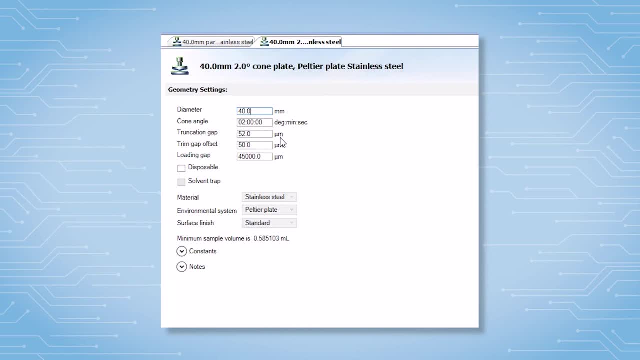 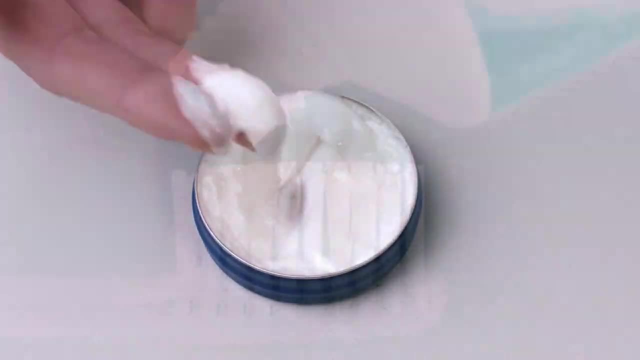 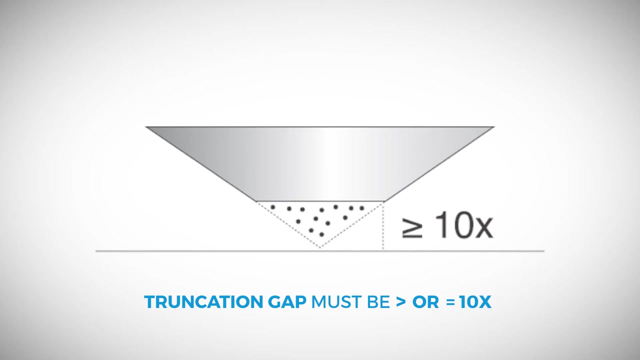 small deviations in the gap height can cause significant errors. A variety of samples may be tested with these geometries, including gels, creams and polymers, Lotions, toothpaste, as well as many others. For samples with particles, the truncation gap for the cone must be greater than, or equal to, 10 times the 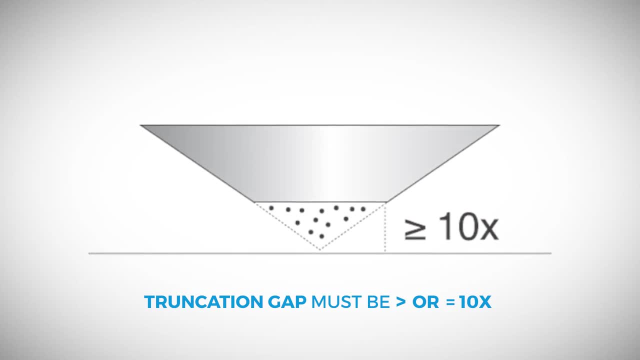 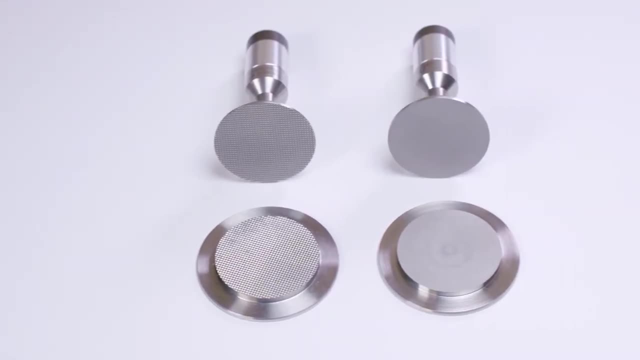 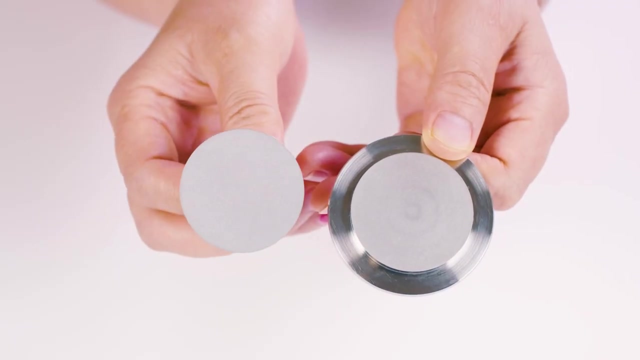 particle size Parallel plates can accommodate larger particles because the gap height may be increased. For samples that exhibit slip, we offer parallel plates with roughened surfaces to help mitigate slip. These surfaces include cross-hatched and sandblasted. For thermostates and samples that cure, we offer disposable parallel plates which can: 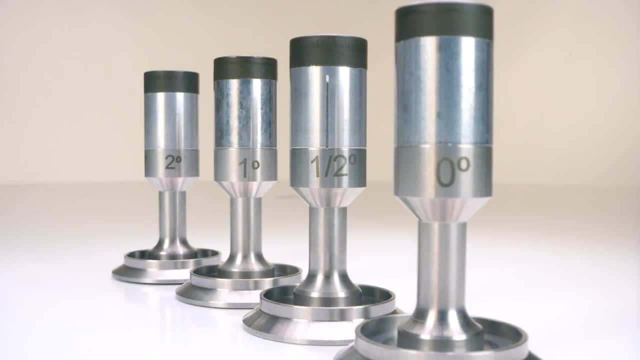 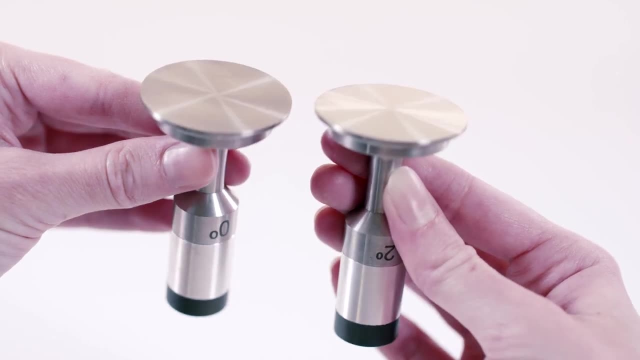 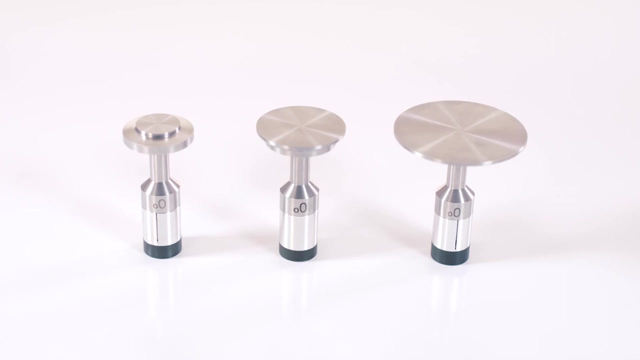 be removed and disposed of after experiments. Next are a few tips for managing torque limitations: increasing the shear rate and selecting a geometry based on sample size. If the torque is too low, consider using a larger diameter geometry, and vice-versa. 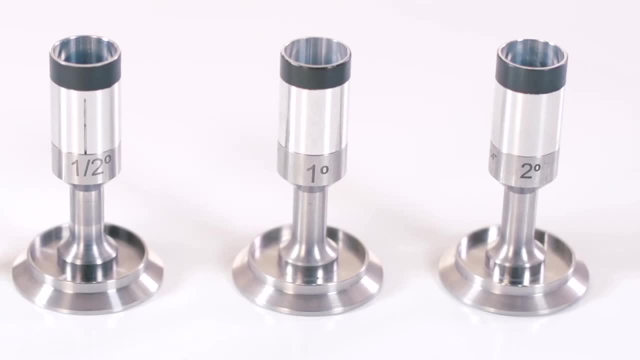 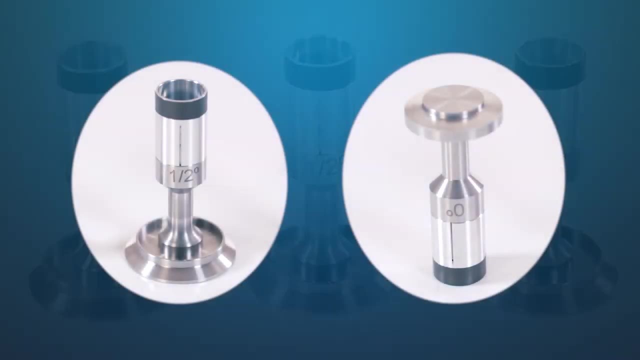 for torque values that are too high. To achieve higher shear rates, use smaller gaps with the parallel plates plate and lower angles with the cone and plate. If you have small volumes of sample, consider using smaller diameter geometries and lower cone angles.